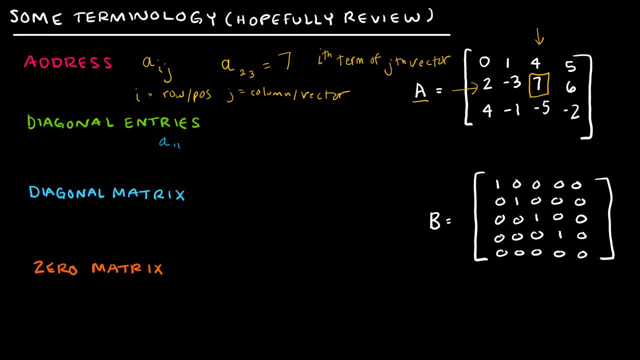 We know what a diagonal is. Diagonal entries would be those in row 1, column 1, row 2, column 2, row 3, column 3, etc. And so in this case, I really only have the 3.. 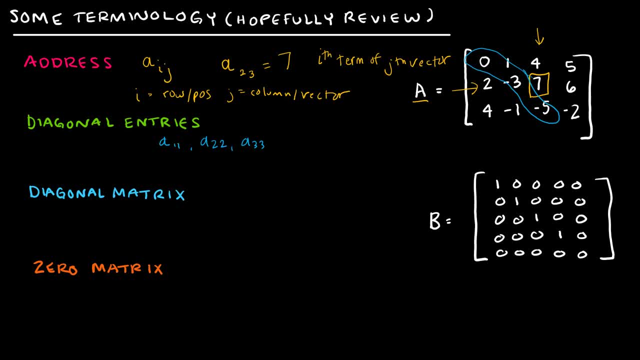 And quite often we don't talk about the diagonal entries unless you're dealing with a matrix A, And quite often we don't talk about the diagonal entries unless you're dealing with a square vector. So I didn't write down square vector as a term, I guess, because I figure it's pretty straightforward. 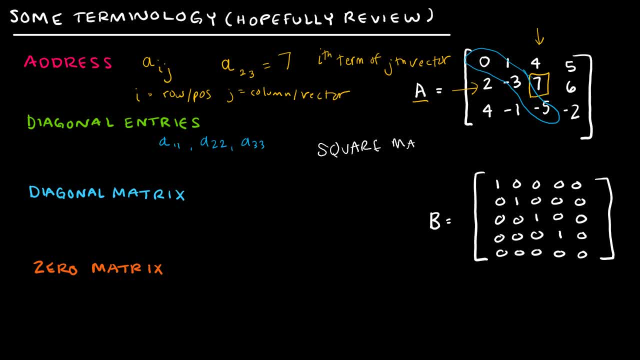 I'm sorry, a square matrix, not a square vector. So square matrix obviously refers to a matrix that has the same number of rows as columns. So a square matrix is n by n as opposed to n by m, which could be any two values. 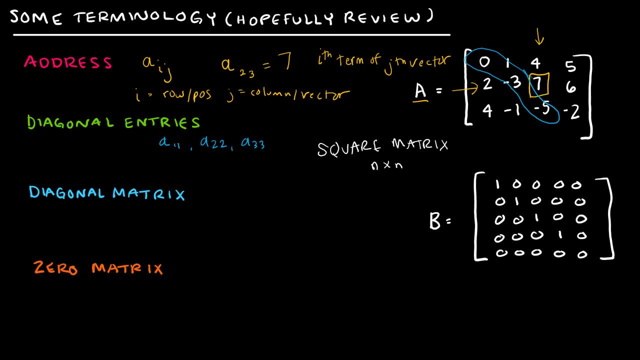 A square matrix has to have the same number of rows and columns. So B, for instance, is a 5 by 5 and therefore is a square matrix. So it's very clear looking at matrix B that we do have a diagonal here. 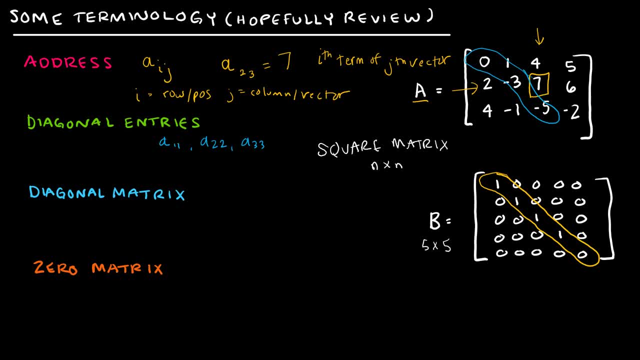 And when we're talking about the diagonals of a matrix, we're always talking about this diagonal and we're not ever talking about this diagonal. A diagonal matrix is a matrix- a square matrix- in which all of the non-diagonal entries are zeros. 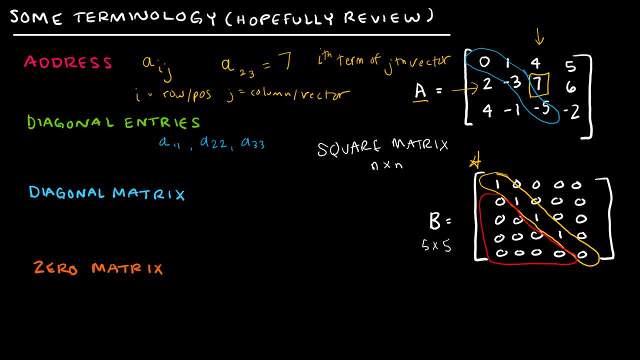 So I'm speaking about, these terms are all zeros and these terms are all zeros. So, as we can see, matrix B would be considered a diagonal matrix. And another term that I didn't put on here that I probably should have is the identity. 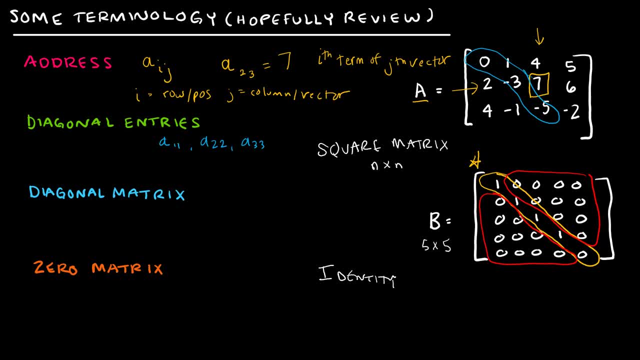 Identity matrix. And again, we've already talked about the identity matrix before, But the identity matrix is where I have a diagonal of all ones, So I would have to change this guy to a 1. And anything that's not in the diagonal would be zeros. 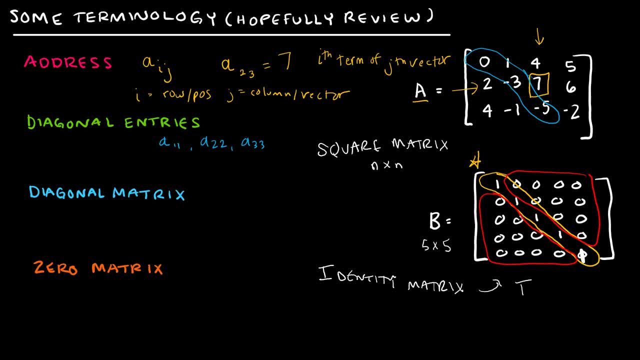 And so this would be the identity matrix for a 5 by 5 square matrix. And then, of course, we already talked about diagonals, And again we're not talking about the diagonal matrix. A zero matrix is just a matrix of all zeros. 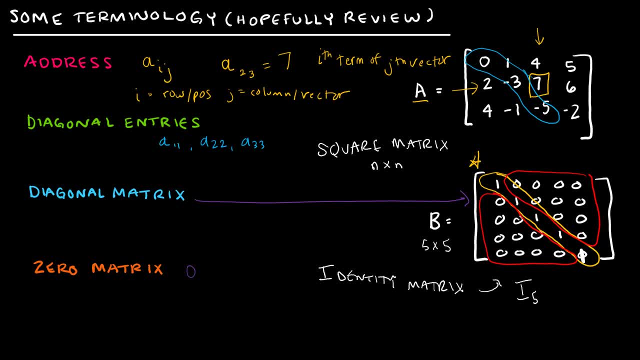 So that one's pretty straightforward as well. We denote that with a zero, And again identity matrix: we denote with an I And then the subscript of however many entries, rows and columns there are. Let's take a look at matrix sums. 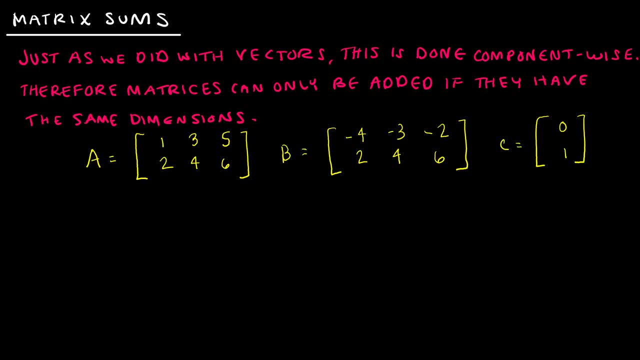 So, just as we did with vectors, when we were adding vectors together, we just added the specific components, Meaning, if it's in the second entry, then we added it in the second entry, And then we added it in the third entry, And then we added it in the fourth entry. 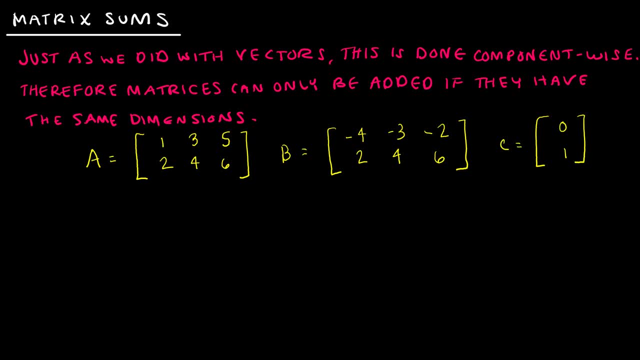 And then we added it in the fifth entry, Then we added it to the other second entry, And so on. So therefore, matrices, just as vectors were, can only be added if they have the same dimensions or exactly the same number of rows and exactly the same number of columns. 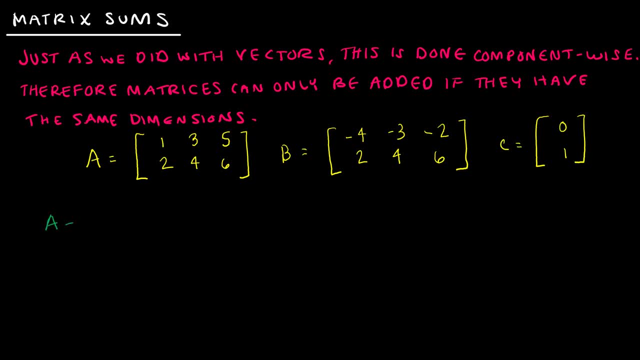 For instance, if I wanted to take A plus B, A is obviously a 2 by 3 matrix, B is a 2 by 3 matrix And therefore they can be added together because they are the same dimension When we say: come on. 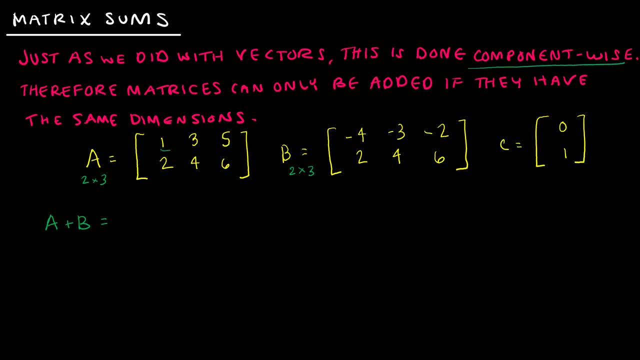 Component-wise, we're saying: take the first entry plus the first entry, So 1 plus negative 4 is negative 3.. And the second entry plus the second entry, 3 plus negative 3 is 0.. And then 5 plus negative 2 is 3.. 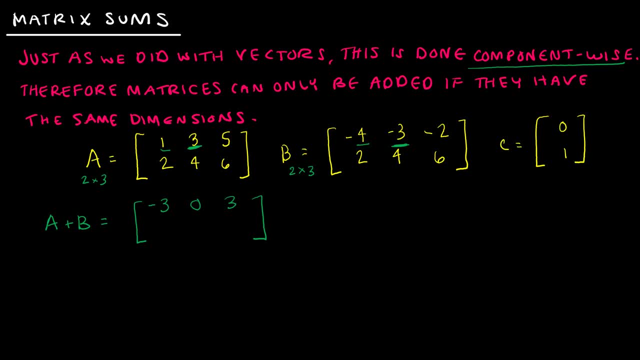 And then the second row. exactly the same way: 2 plus 2 is 4.. 4 plus 4 is 8.. 6 plus 6 is 12.. Just like that, A plus B, And of course, if we said find B plus A. 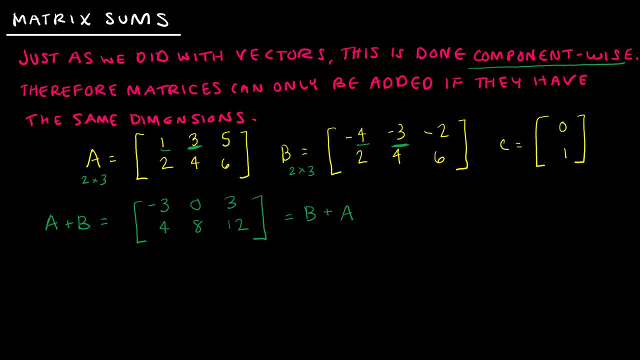 That would be the same as well, because it's addition And therefore commutative, and would give us the exact same solution. If I said let's take A plus C, We would say that's not valid Because C is obviously a 2 by 1.. 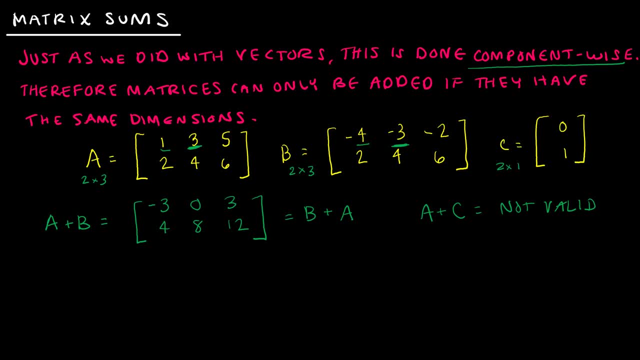 So it's a column. vector A is a, 2 by 3. And those are not the same dimensions. Similarly, I could not also find- Excuse me, not A, But B plus C would also be not valid. Now, keep in mind that we're talking about matrix sums. 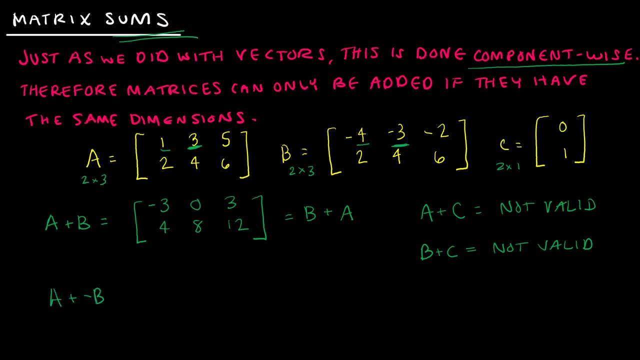 But if I said: take A plus negative B, That's really just like A minus B And we can totally do that And you can think of it either as A plus negative B, Meaning go into- And I'm going to change colors here for clarity. 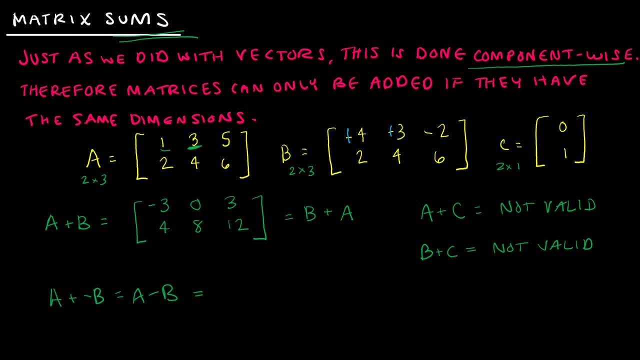 Go into matrix B And change all of the signs And then add them together. So 1 plus 4 is 5.. 3 plus 3 is 6.. 5 plus 2 is 7.. And then 2 plus negative 2 is 0.. 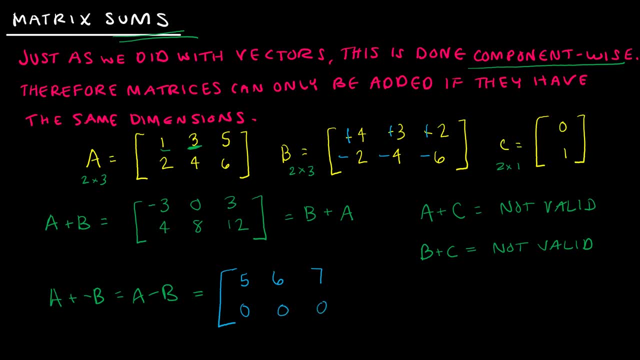 4 plus negative 4 is 0.. 6 plus negative 6 is 0.. So that's one way to think of it And of course the other way is just to subtract And hopefully, if you are in linear algebra, 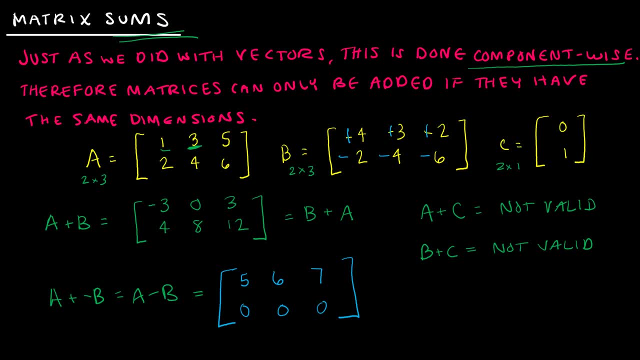 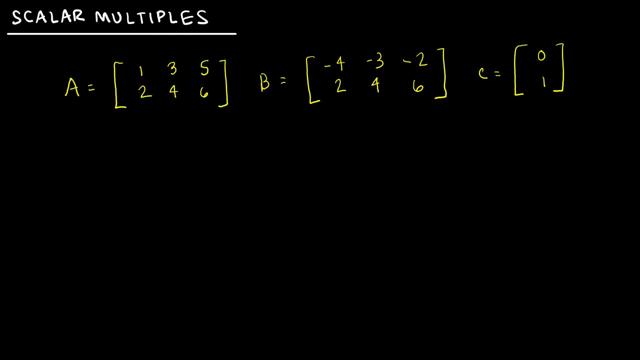 You're able to subtract with negatives Without mixing up your signs. We've also discussed before scalar multiples, And we did this when we were dealing with vectors. But it's the same thing Whether it's a vector or a matrix. So if we're dealing with a scalar multiple, 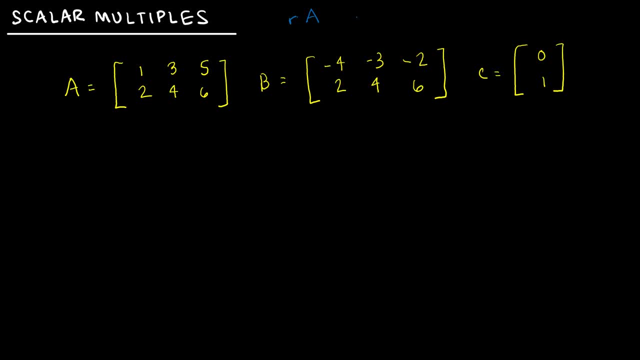 That means I have something like R- A, Where R is my scalar And A is obviously a matrix. So typically I would have something like 2- A, Which just tells me to take 2. Times each entry in matrix A, So it's just telling me to double. 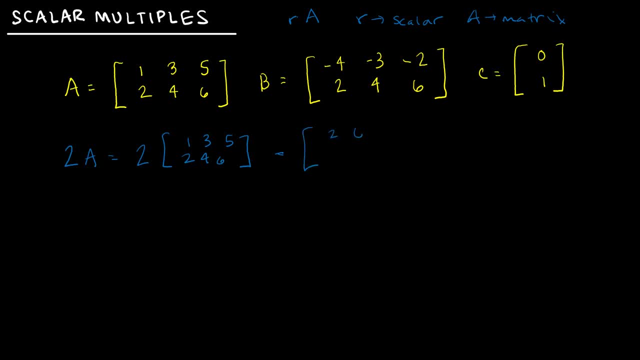 And again it's just each value. So 2, 6, 10.. 4,, 8,, 12.. And there's my solution. I could also have- And this is more typically what happens- 3 A. 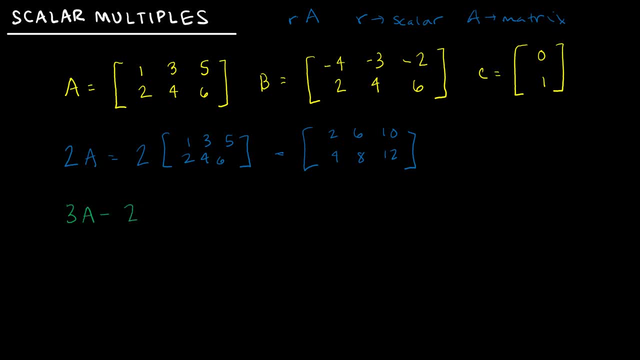 3 A Minus 2 B. So in a situation like that I would take 3 times A And notice I am showing all of the steps. So it's very tempting to just Write the solution. That's not a good idea. 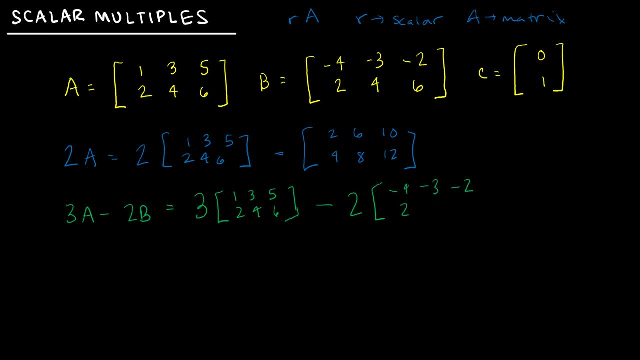 Unless your instructor says it is, And I am your instructor And I am saying: hey, Show work, Unless I tell you otherwise. So again, take 3 times everything in A: 3,, 9,, 15,, 6,, 12,, 18, and then it's your choice how you. 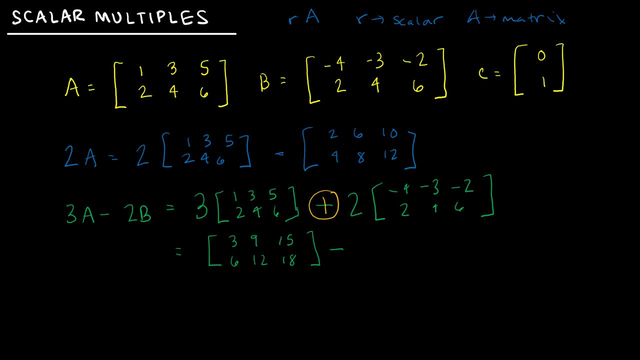 want to handle this negative, So a lot of people go ahead and make this plus and turn that into a negative 2. So then my solution or my resulting matrix would be negative 2 times negative 4,, which is 8, and then 6, and then 4, and negative 4, negative, 8, negative. 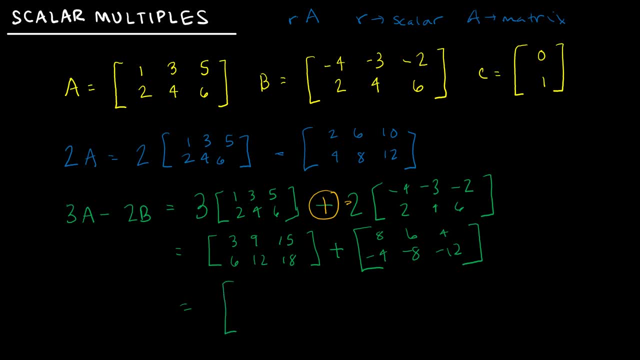 12.. And then I'm just going to add those together Again. we just talked about addition and that's component-wise. So 3 and 8 is 11,, 9 and 6 is 15,, 15 and 4 is 19, and then 6 and. 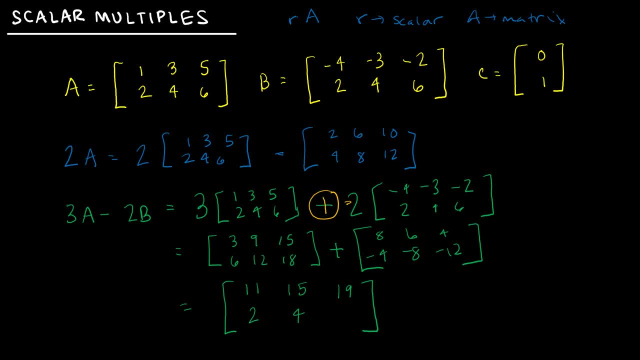 negative 4 is 2, 12 and negative 8 is 4, 18 and negative 12 is 6.. And that would be my solution. Notice, I didn't use C in this one, but C would be exactly the same. So if I said 3C, it would just say take 0 times 3 and 1 times 3, and that's my 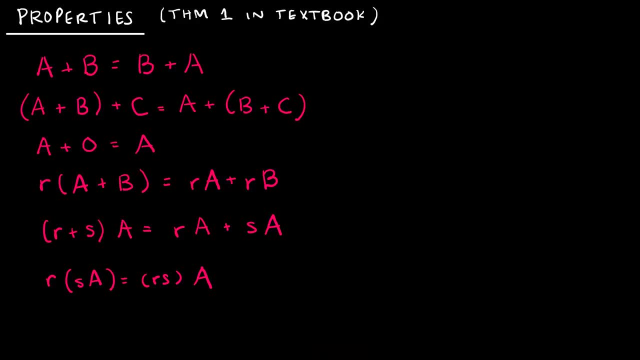 solution. I'm going to quickly go over this page, but these are properties that you should have been familiar with since you took Algebra 1 for the first time. So, yes, these are dealing with matrices A, B and C and scalars. 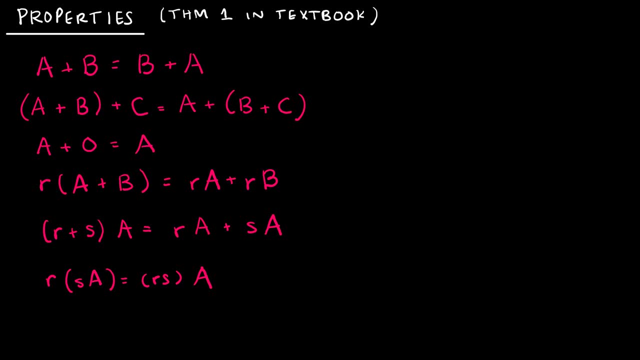 But really, if you look at that first one, this is just the commutative property of addition. If you look at the second one, that's the associative property of addition And yes, we're dealing with matrices, but it's still the same property. This is the additive identity. 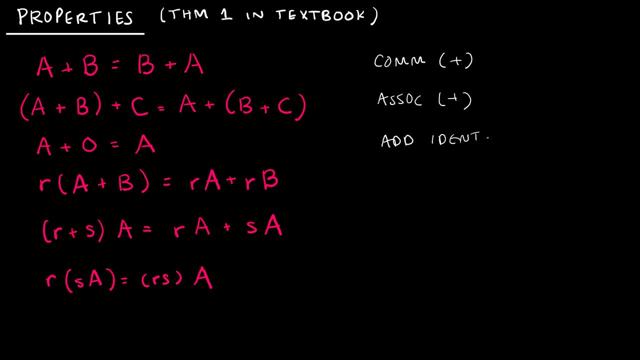 property, which means if I add the zero matrix to any matrix, I end up back where I started. This is the distributive property, as is this, So you can go in either direction on that distributive property And that last one is: 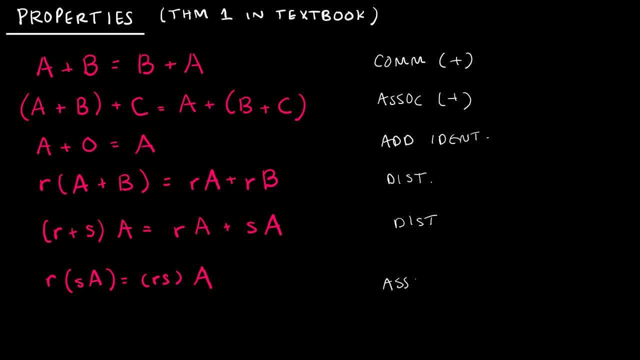 really just the associative property of multiplication instead. So I can multiply in the other order and still. But again, this one's a little bit different because R and S are scalars and A is a matrix. But as you can see, all of those properties hold true. 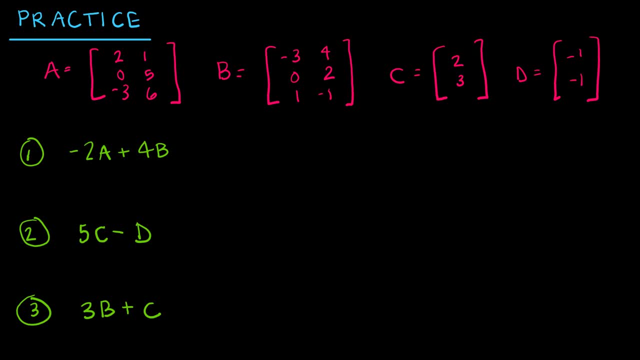 Here's just a bit of practice for you to do on your own. This is dealing with both scalar multiples and matrix addition. When you have tried all three questions, press play to see how you did So. the first one is negative: two A plus four B. So the first thing I'm going to do is verify. 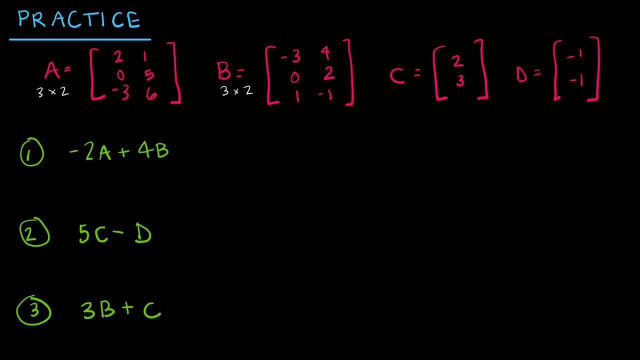 this is a three by two matrix and this is a three by two matrix And a scalar obviously will not change our matrix dimensions. So we definitely can do question one. So question one says negative two A. So I'm going to go ahead and write what negative two A is. 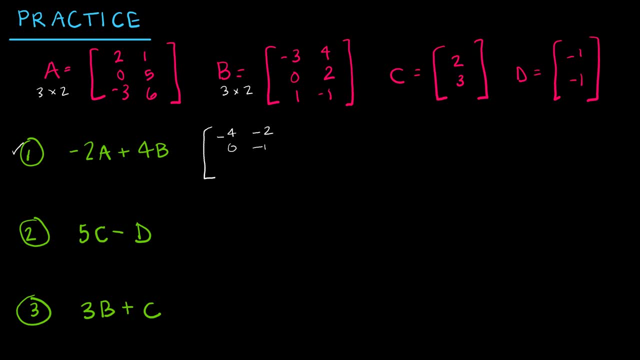 So I'm going to put negative four, negative two, zero negative 10, six negative 12.. Plus four B, So four times negative three negative 12, four times four, four times zero, four times two, four times one, four times negative one. 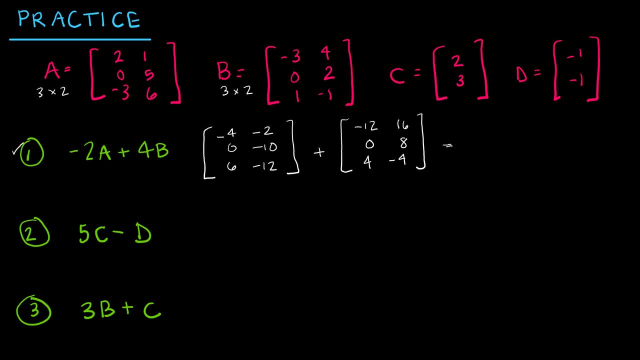 And then my result will be the sum of those two results Resulting matrices, which gives me negative 16, 14, zero, negative two, 10, negative 16.. And then I'm going to look at question two. Question two is five C minus D. Again, C is a two by one, D is a two by one, and so I 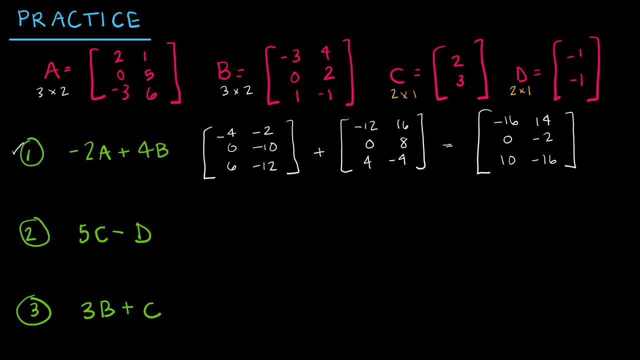 can see that. You see that the operations within those confines will work just fine. So five C would give me 10, 15.. Minus D, which is negative, one, negative one, And again it's up to you how you choose to deal with minus or negative. 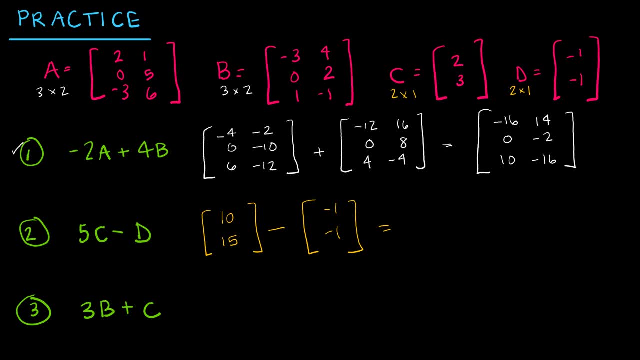 Uh, 10 minus negative one. A lot of people just make that plus and then change the sign of every term in the next matrix, But that's completely your business. So 10 plus one minus D, That's negative one. that's negative one. 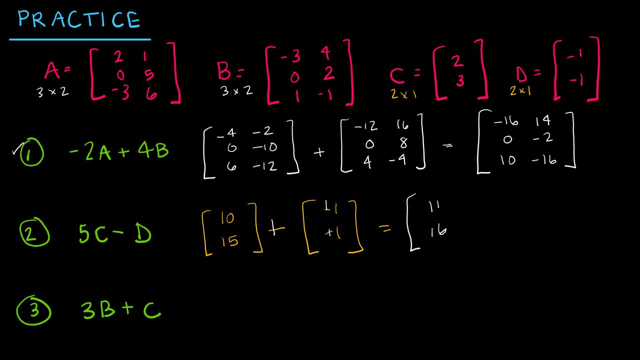 1 is 11.. 15 plus 1 is 16, and there's my result. Last one: 3B plus C. B is a 3 by 2.. C is a 2 by 1.. This scalar is not going to change that, so this is not valid.